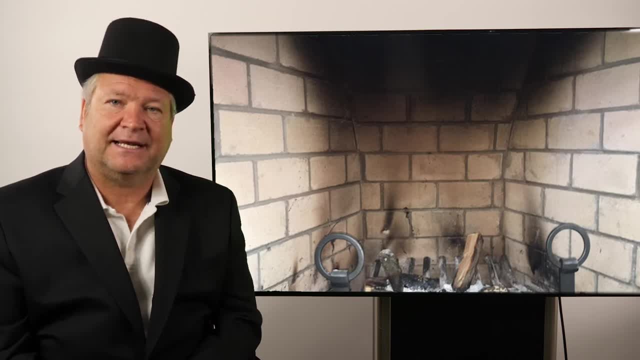 it says: you know what? The brick joints have got to be a quarter inch thick and it's got to use ASTM refractory mortar. All right, what does that mean? Here's what it means. Back in the old days, they used to use a quarter inch thick brick joints And they used to use a quarter inch thick brick joints. 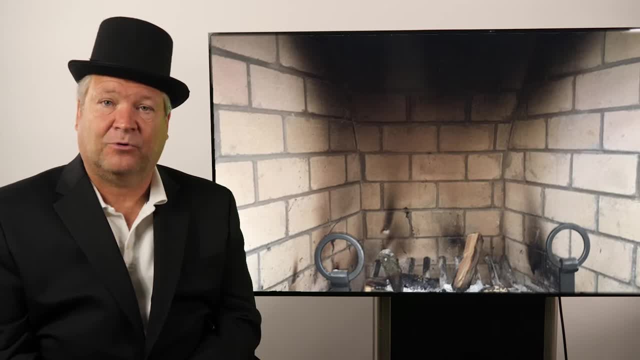 низ. Orlando did not die of a heroic sunrise, Did not kill people in theapper- that they are sure Con tint. they used to make line mortar. They used to make chimneys all the time and they would use lime mortar. Line mortar's great. it's called hydraulic mortar, Anyway. so then they changed to this thing called Portland cement, but that was around 1900. And then they started making. 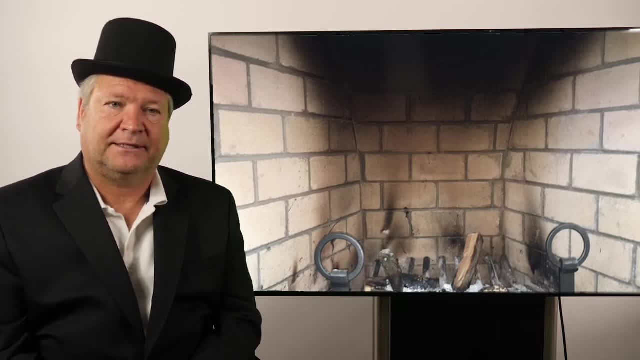 And then they started making mortar out of Portland cement. Well, guess what? Portland cement just doesn't do very well in high temperatures. It's actually it doesn't do well in high temperatures. it goes up to a certain amount and then, as it cools through about- oh, maybe 600 degrees Fahrenheit, it starts breaking down. 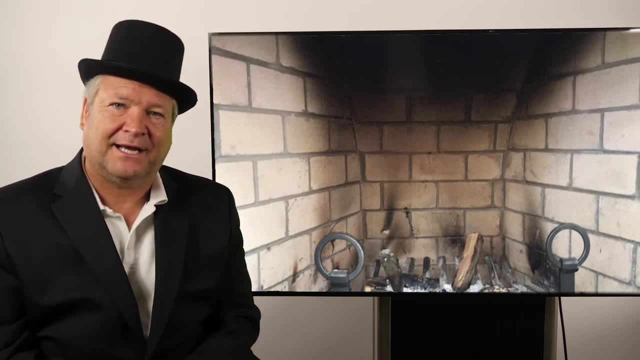 So it was, like me, the only guy that ever evangelizedт skillset on how. never again it's breaking apart. Go figure, You wouldn't know. So building codes now call to have refractory mortar and a quarter-inch thickness. I think what they really want is is that they want the 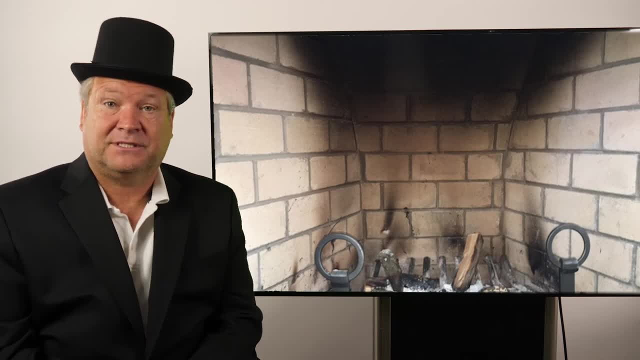 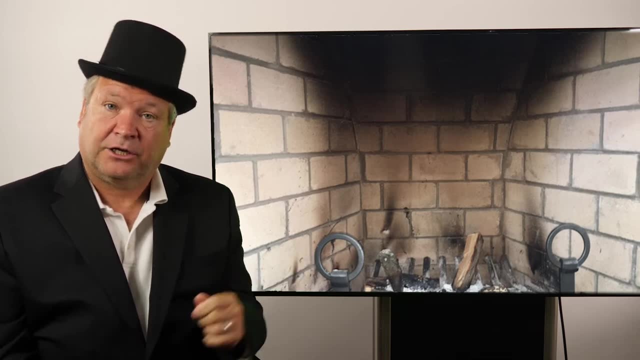 refractory mortar. It doesn't matter about the quarter-inch thickness, All they know is that there's mortar joints that are failing. So how do mortar joints fail? They fail one because of water. You get water come down, get inside of these mortar joints that are already deteriorating. 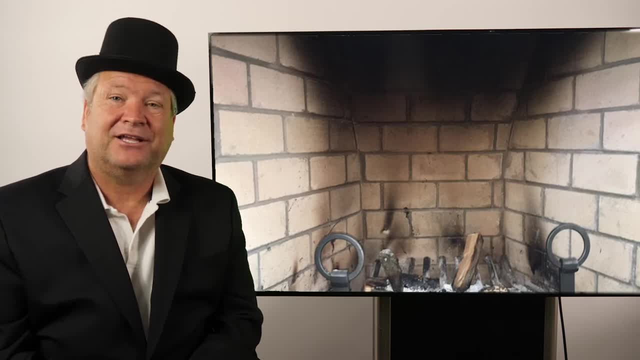 and it causes problems. Two, they're not using refractory mortar. They're using regular fire clay inside of regular mortar. Now there are ASTM-type mortars and there are some that use Portland cement inside of these mortars, But what they use is is they use these special? 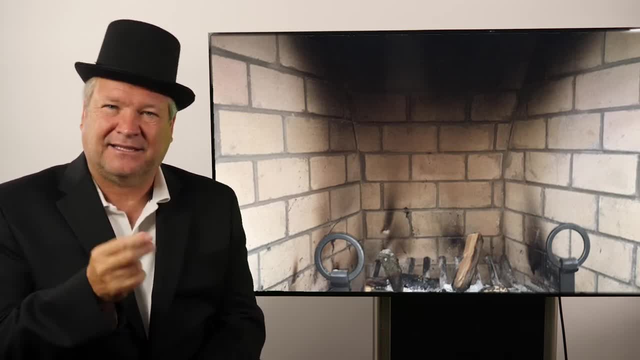 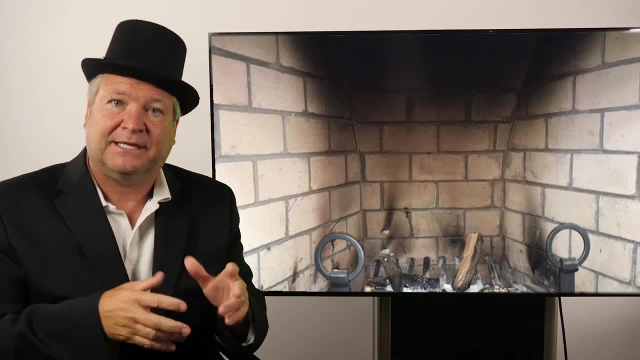 aggregates. What's an aggregate? An aggregate's like the sand and the little pebbles and things like that that goes in it to make up the mortar. So it's got the cement, special aggregates and all the other items And what ends up happening is is that if you use this special 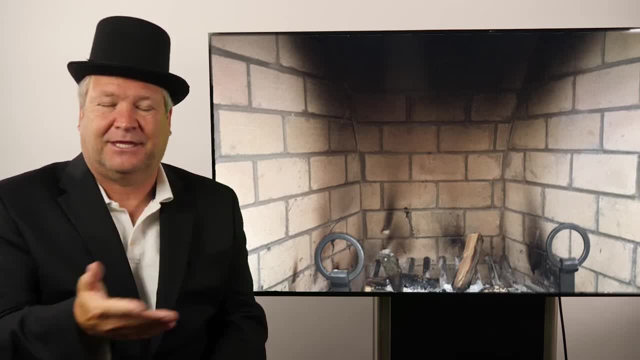 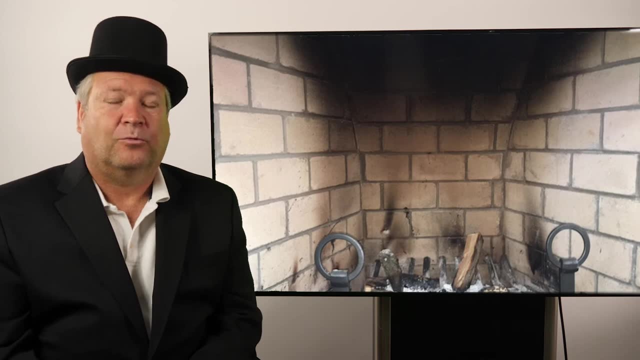 stuff, then it won't break down as it drops under the 600-degree Fahrenheit temperature. That's called ASTM-C199 type of mortar. What does that mean to you as a homeowner? It means this: If you're looking at your fireplace and you see there's a bunch of deteriorated mortar joints,